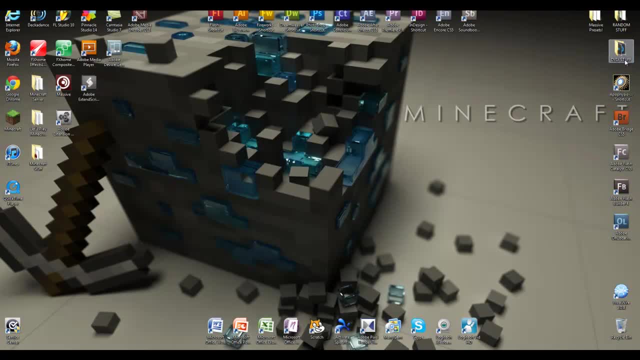 Hey guys, welcome to this new tutorial on my other channel. As you guys see the title, I'm going to show you today how to use this cool little software- it's free software- on how to make fractals, And if you don't know what fractals are, they're really cool. digitally produced, I really don't know. they look like light renders. they look kind of like cinema 4D renders, except they're kind of like light, you're. why don't I let you see for yourself? 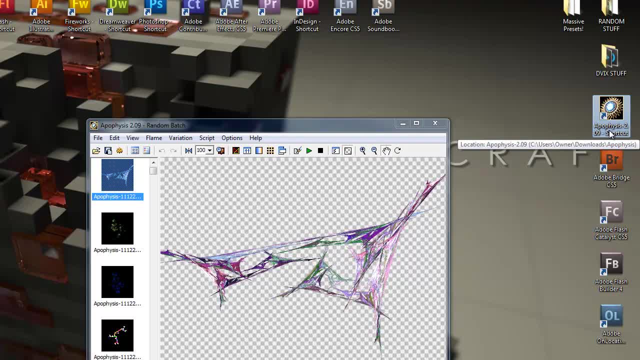 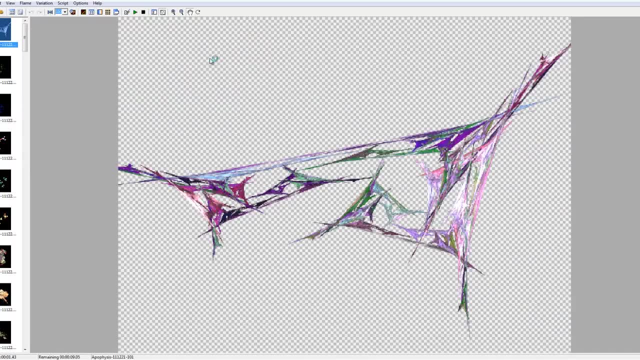 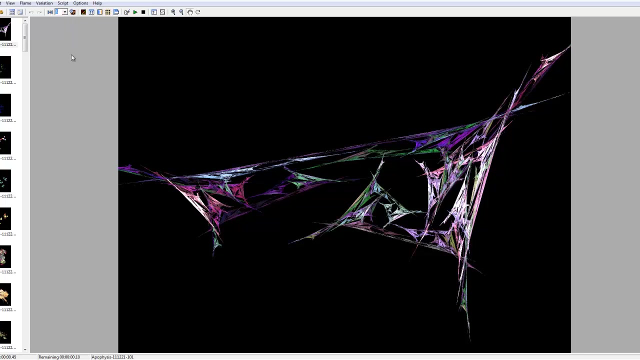 So I'm going to open up this program called Apophysis and, as you can see already, this little image on the screen looks pretty cool, So let me just Put that there. it's kind of so. first thing you want to do is, if this is clicked on- that's the transparency- click it to black, just because it gives you a better view, and if it's off, and make sure you change this little drop down menu to 5, just so it renders faster, because it'll take a little while. 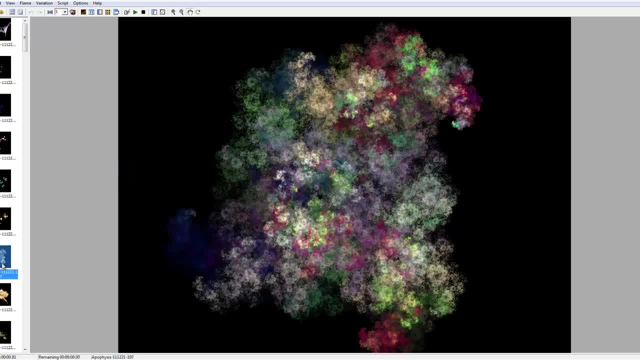 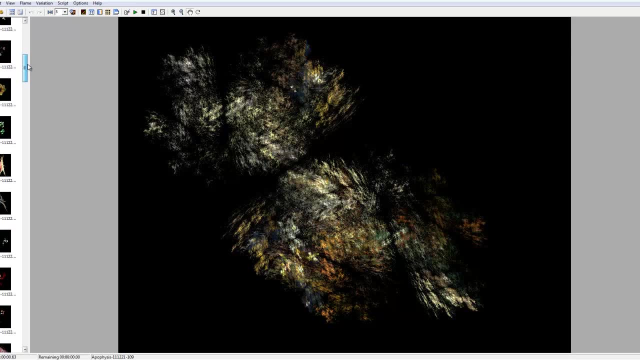 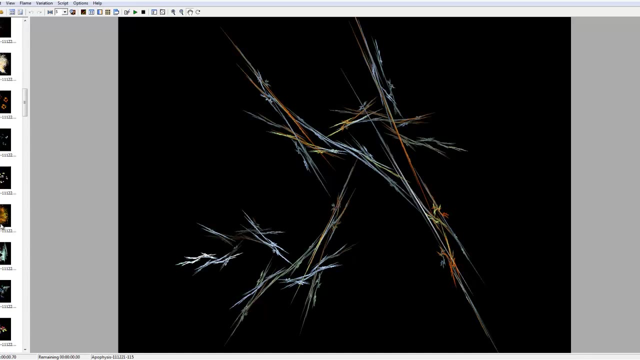 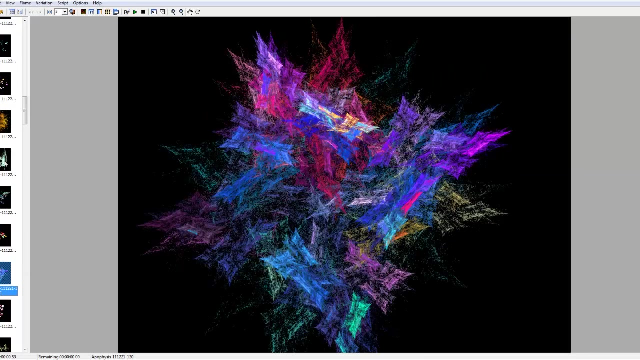 So now just put on one of the demos over here in this window over here, you'll see there's a whole bunch of like, pre, Pre, like, rendered out different. they're called flames. that one's cool. I like this one okay. 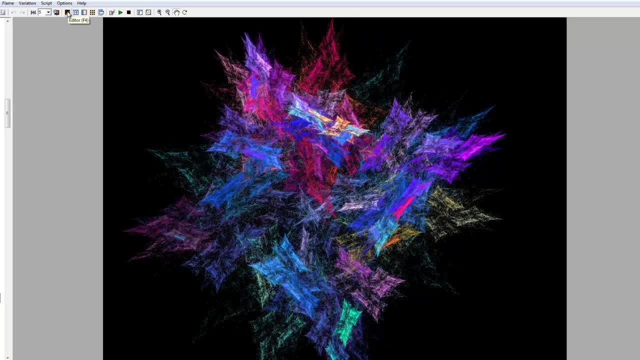 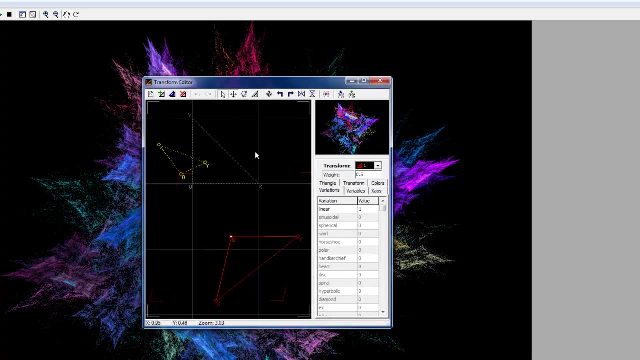 So now what you're going to want to do is this little button over here is called the editor. open that up and you're going to get something like this pop up. Now don't get mad at me, because I'm not completely like fluent with the software. 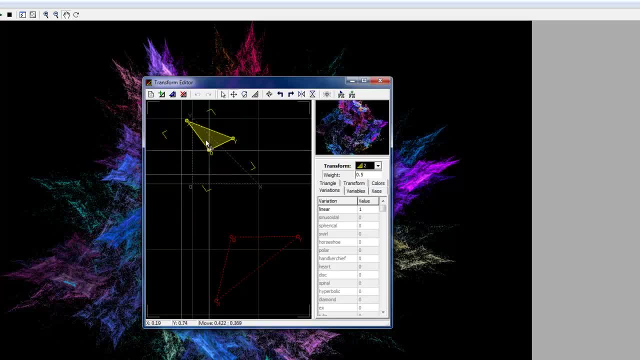 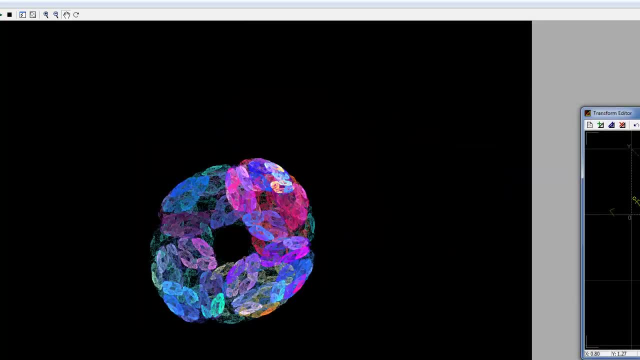 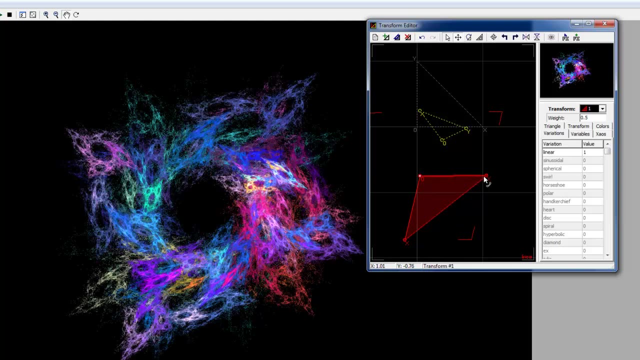 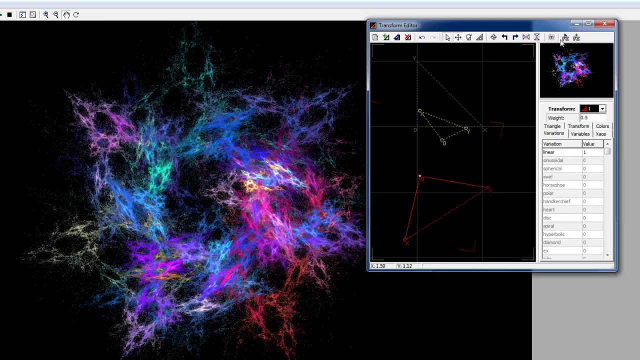 I just know the basics. so basically, what you do is you can drag these triangles around, make a big donut shape. I'll move this over here so you can see what's happening on the screen. That's pretty cool, Alright. so now, now that you've got a nice shape, now why don't we go over here? 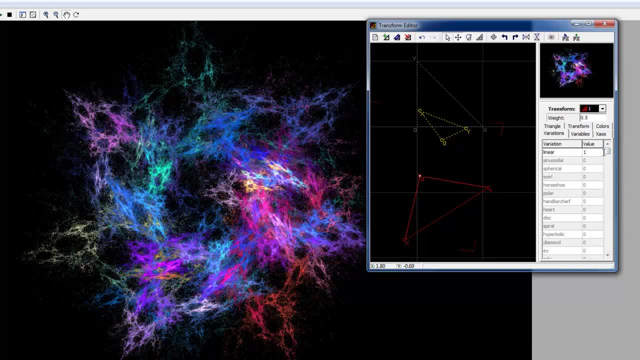 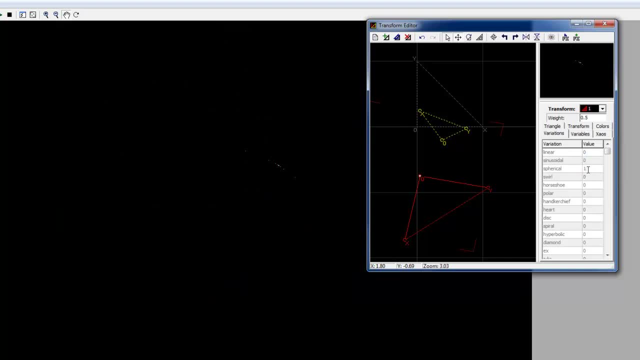 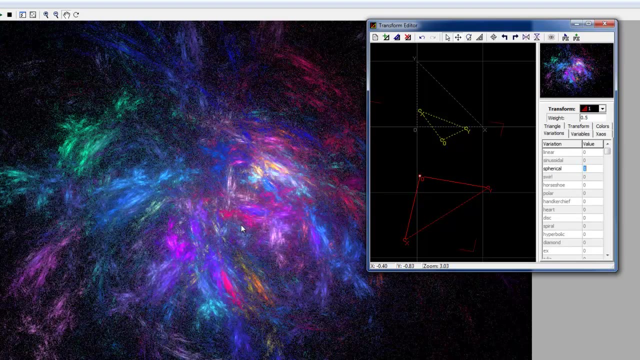 So this little panel, make sure you're on the variations tab, change the linear to 0, and the spherical to 1, press enter. So, as you can see, something pretty cool happens this. um, now, all these things, all these little variations, there's like 100 or so, maybe not 100,, maybe like 50.. 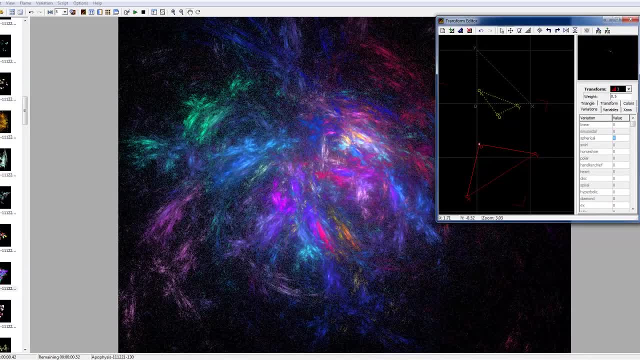 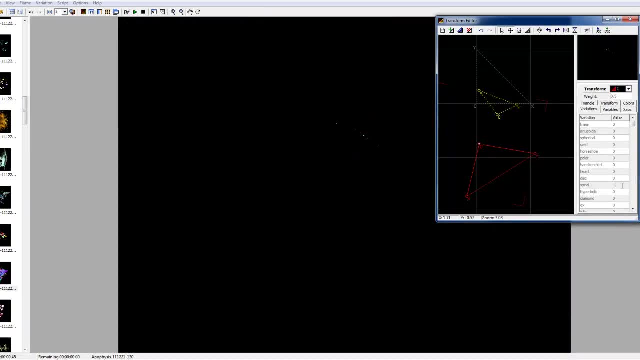 Okay, let's just play around with this. So I'm going to move this down a little bit. so change that back to 0, and turn on the spiral. turn that on to 1.. You never, ever want to do one or more, because I'll show you what happens. 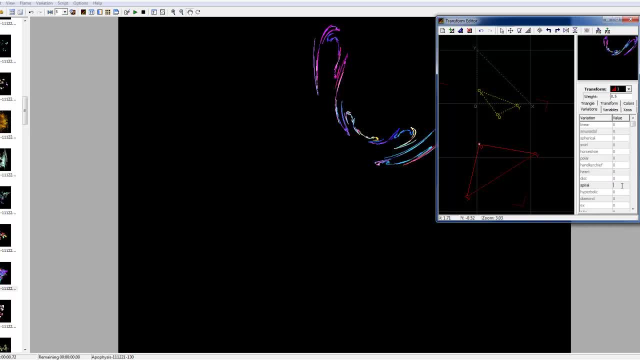 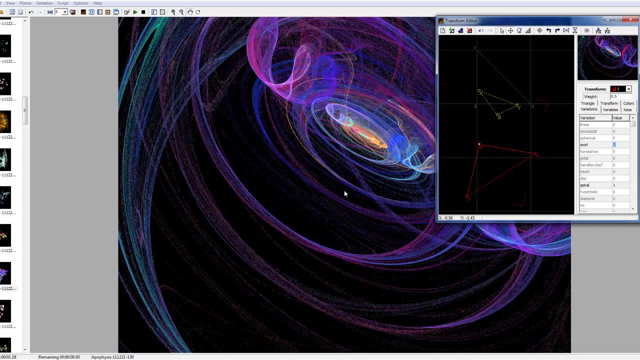 Um, oh yeah, I forgot to put that in present, So that's what happened. Alright, now let's put on swirl 30. See, it's hardly visible because it's even 2 is like doesn't really do it justice. 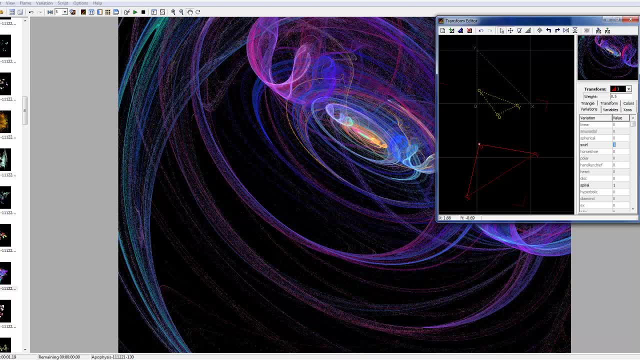 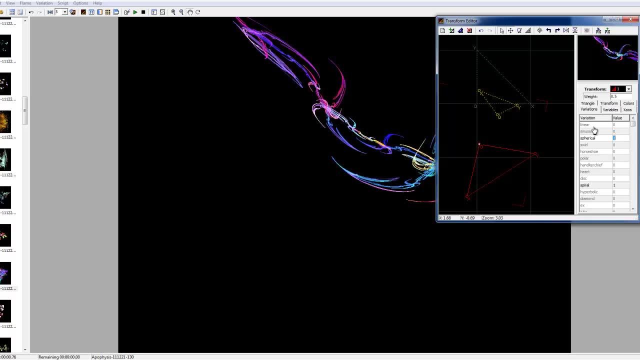 So, oh, that that's pretty cool. So that's the spiral function. Change that back to 0.. I like the spherical one, so I'm going to put that back on 1.. So you only want to change it to 1, because any more than that it gets weird. 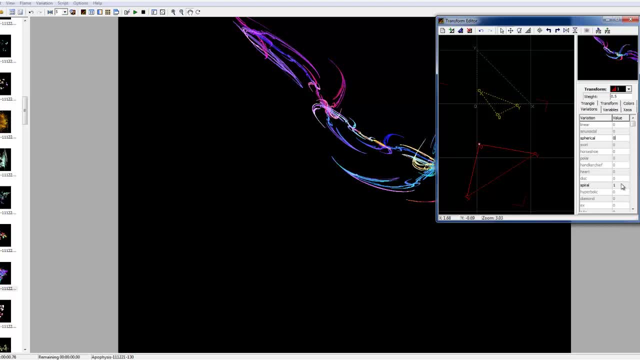 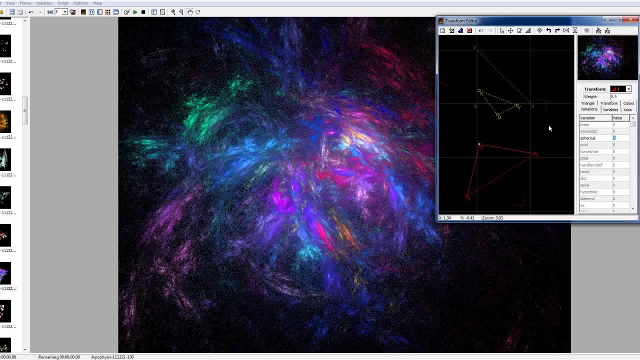 Actually, no, never mind. spherical is kind of annoying. Um, oh, I think I know why: Because I have spiral on. Pardon me. Alright, there we go. So now you've got the right like um shape that you want. 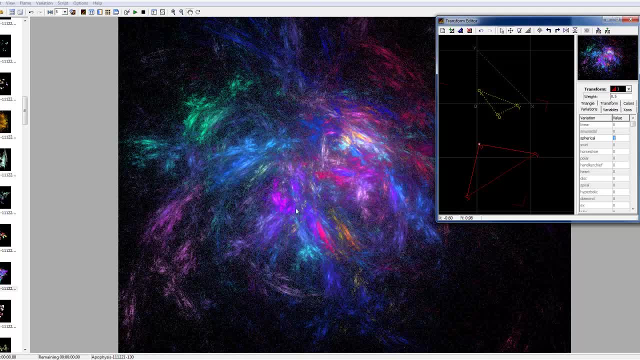 Um, but you don't like the placement of it, you don't like where it is in the screen, So we're going to just use that. You can do it one of two ways. The first way is by clicking Effects, and this creates a new triangle. 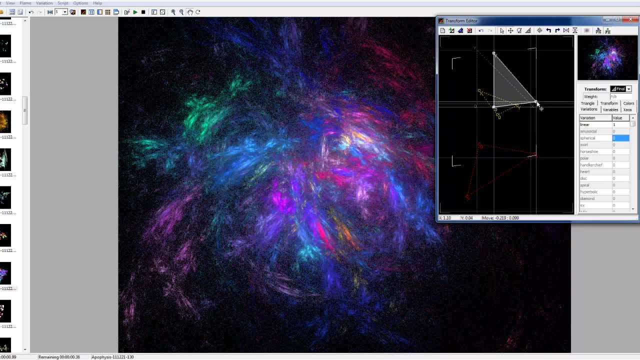 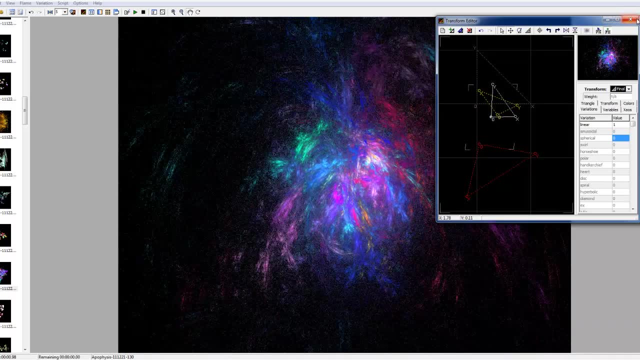 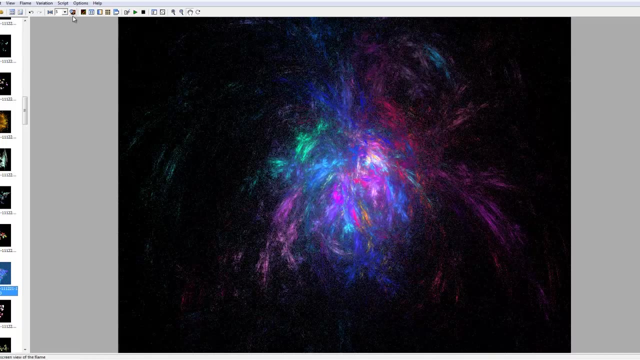 And you can move it, this triangle, around, resize it however you want, And there you go. Alright, uh, so now you can close that out. after you're happy with the shape of it, You can close that out. Now we're going to open up our gradient. 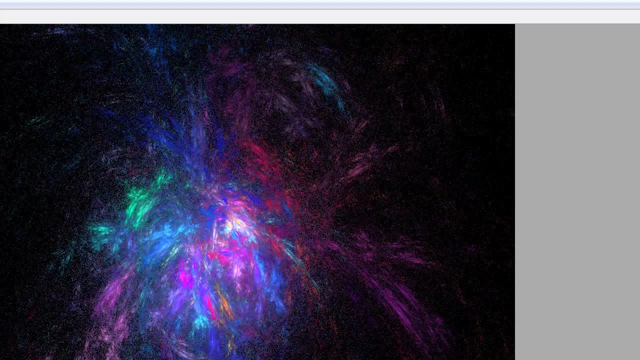 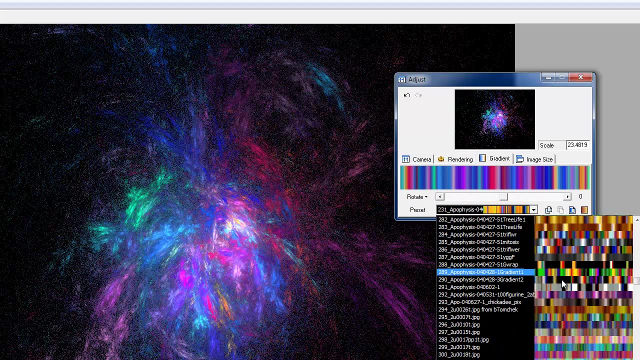 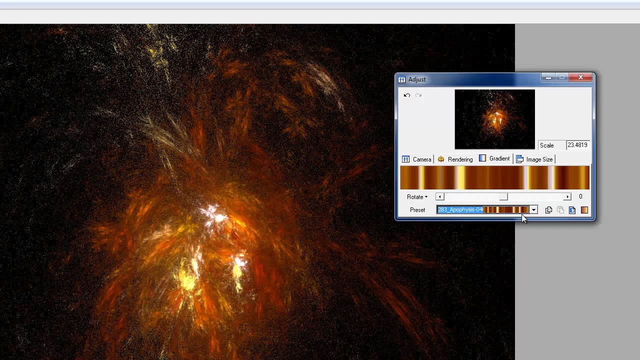 Or you can shortcut F6, opens up this little panel over here. Uh, now this is where you choose the color. So just, there's lots of gradients You can make your own, but for the sake of this tutorial, I'm just going to use a pre-made gradient. 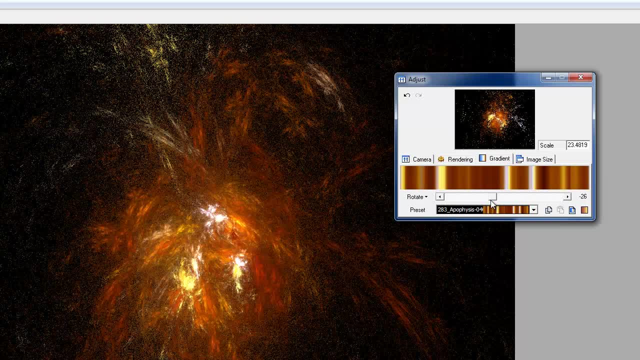 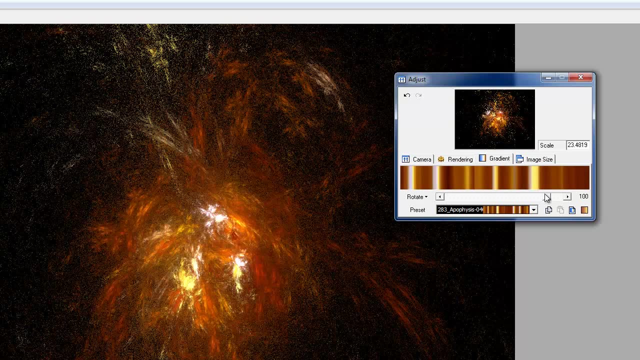 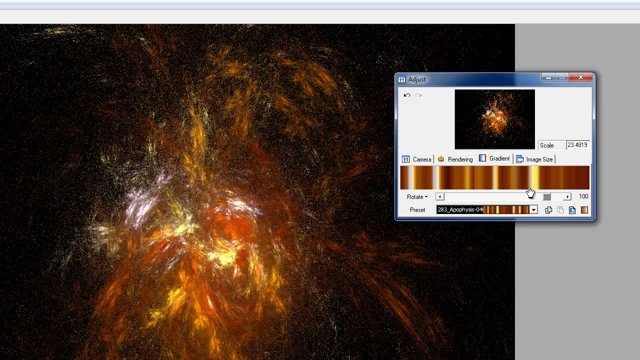 So I like the look of this one. You can use a slider, scroll around see which one you like, And what I'm trying to do right now is get most of the light in the center of this Like that. Alright, so now that you're happy with your gradient, uh, you're going to go over to Rendering. 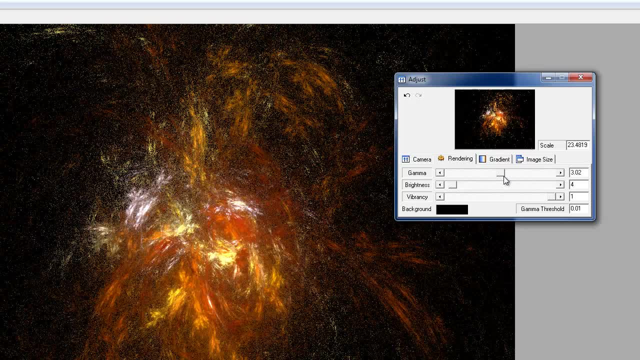 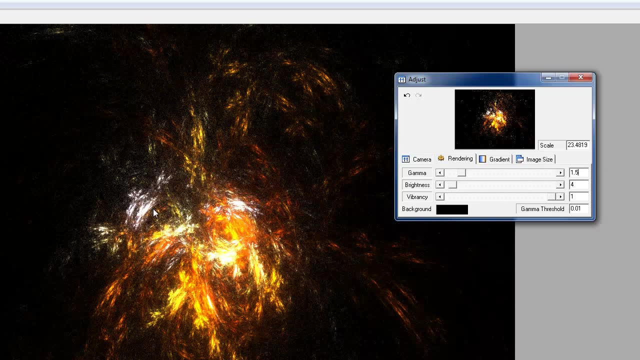 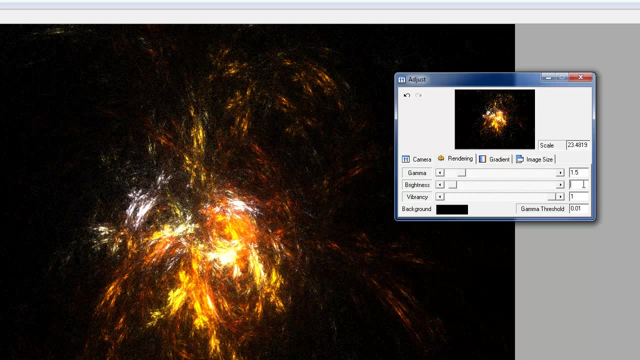 And what I like to do is bring the gamma down to about 1.5. And, as you can see, this just kind of gets rid of all this noise over here and brings out the hot spots. What I also like to do is bring the brightness up to 10.. 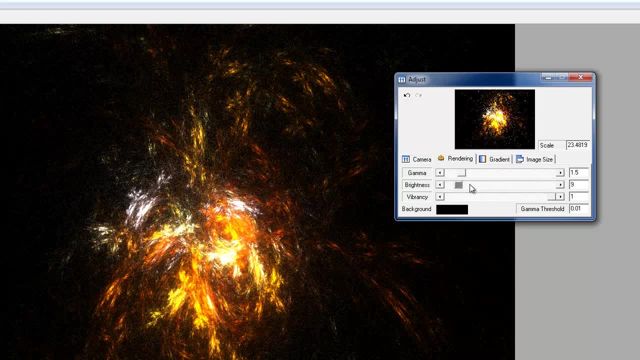 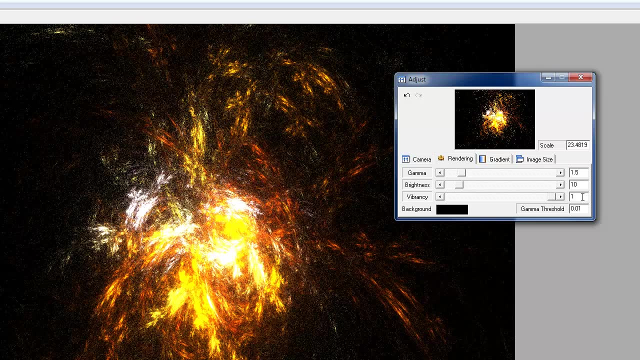 About. you can bring it higher if you want by dragging the slider, And that's cool. So 10, there we go, And vibrancy. you don't want to adjust the vibrancy because what the vibrancy does is it? it's kind of like a saturation. 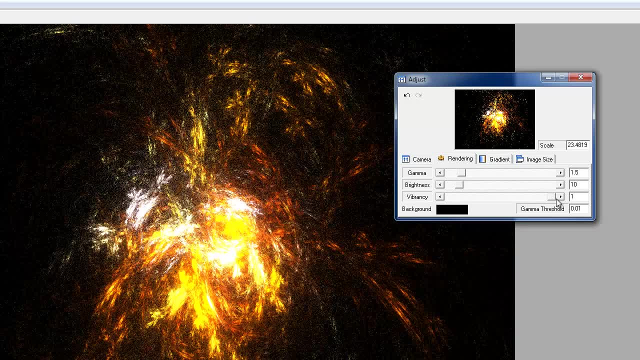 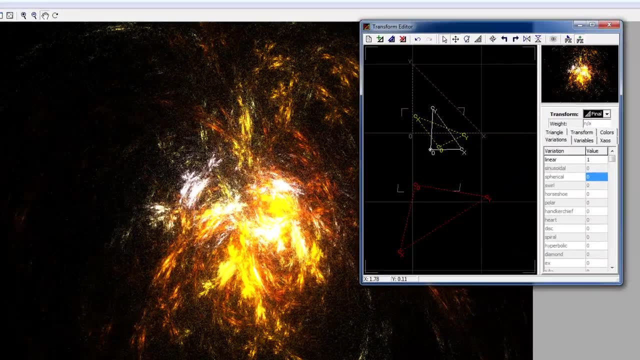 It takes most of the color out of it, So that's why I like to leave the vibrancy all the way back at 1.. Now here's the other way you can move it around. Instead of using the tool, the white square er the right triangle- here you can use the camera tools. 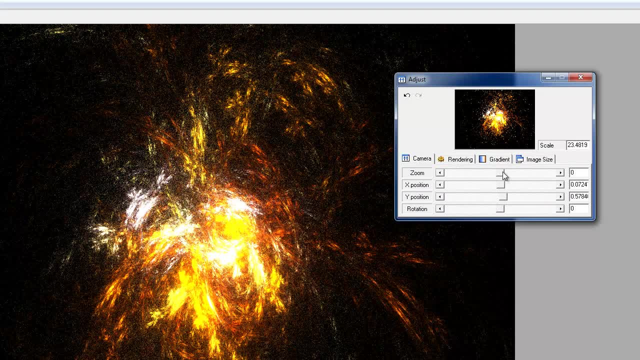 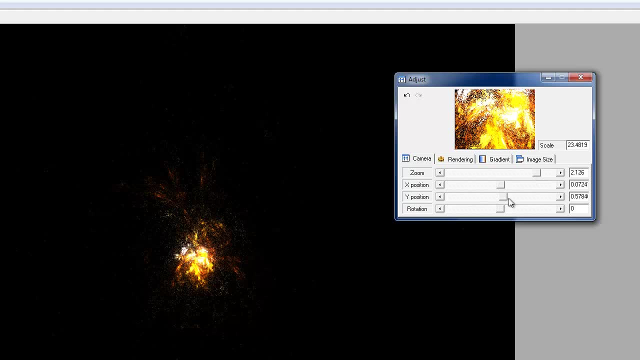 Now, what the camera tools are is basically, you can zoom it in and out. Okay, that's going to take a while. I'm going to just leave it right there, though, because I like it there, Actually, maybe a little bit smaller. 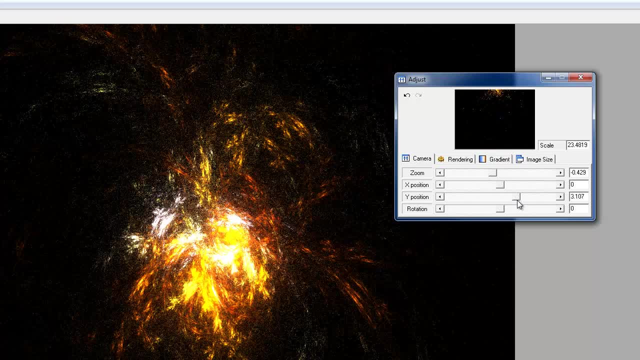 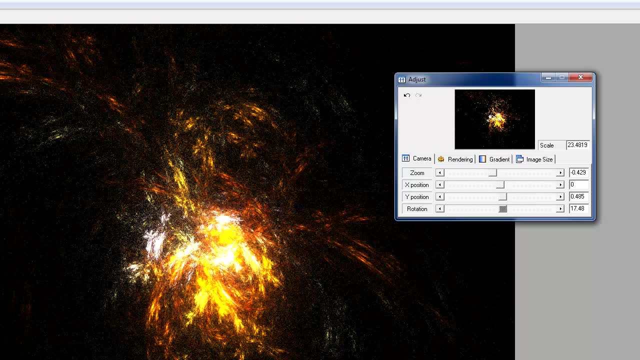 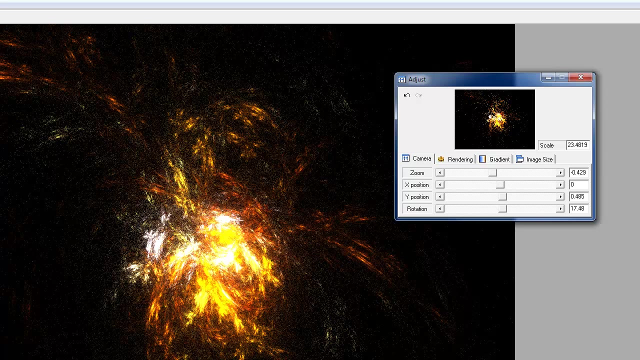 Um, and you can move the X position and the Y position and the rotation. So these tools are a lot easier, in my opinion, than using the white triangle. Oh sorry, Like, oh whoop. Here's a retake. 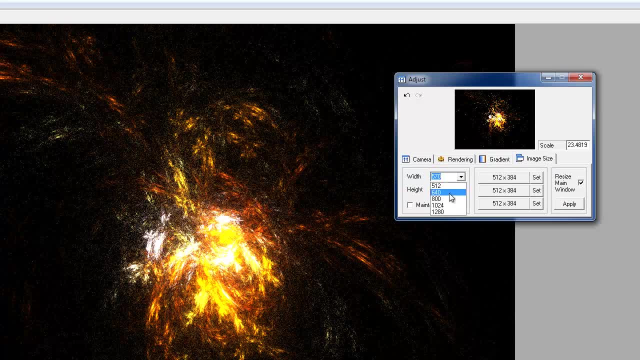 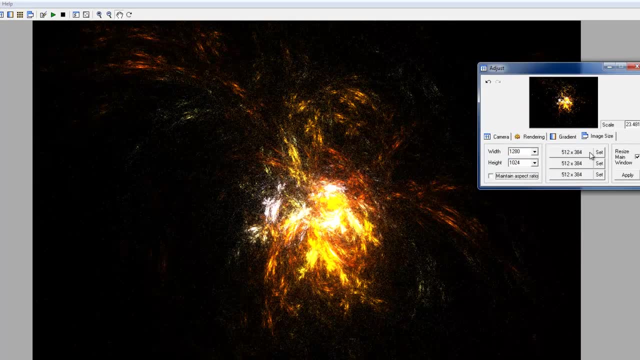 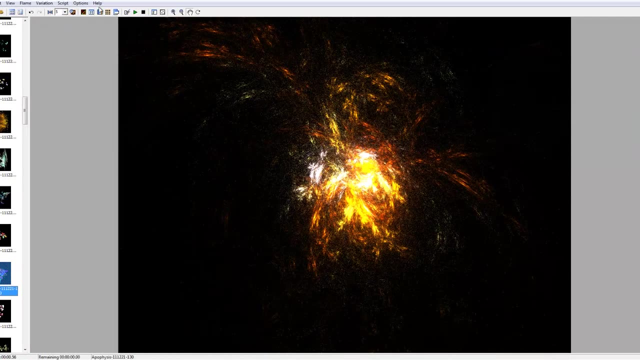 And then, last but not leastly, we have the image size. Uh, I usually adjust it to 1280 by 1024.. Um, just because I like them big, Pardon the pun, So close that out. Uh, and if you're happy with what you have right now, we're going to render it. 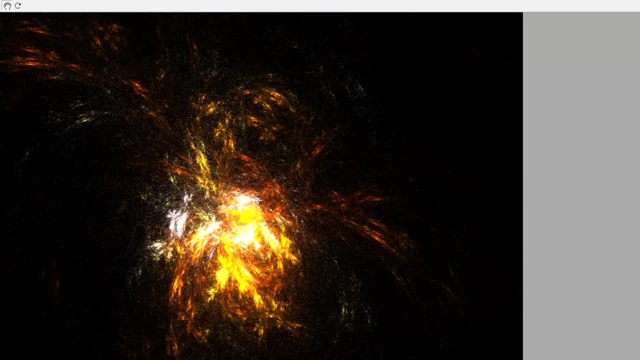 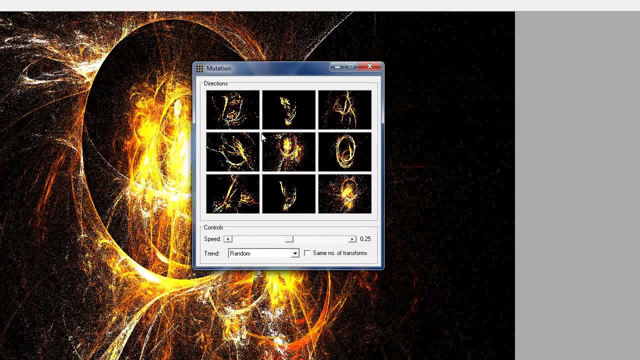 Uh, now, obviously you're going to have to like experiment This. oh, one more thing: The mutation window. You can click on different types of mutations and it'll just like they're basically just randoms. 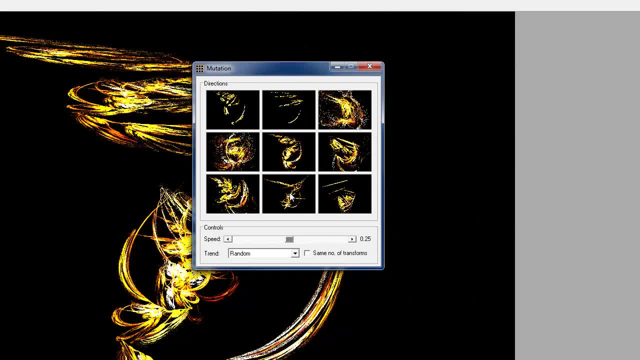 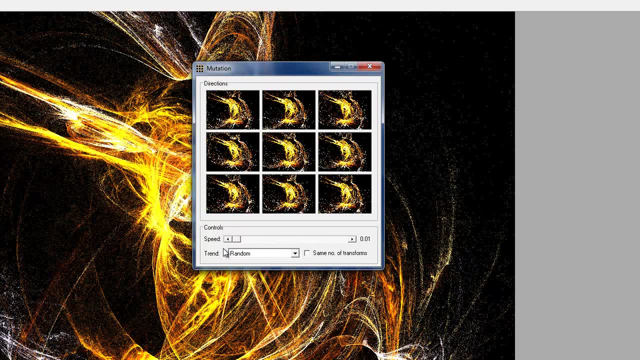 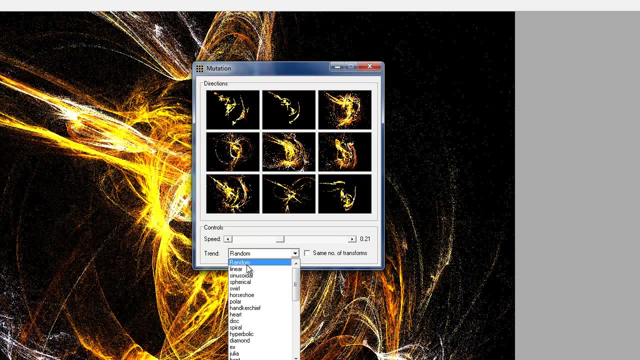 You can do so many cool things with them. So you have that Uh speed. This just adjusts like how drastically And you can adjust the variation. Um, so yeah, I'm happy with this. It looks really cool. 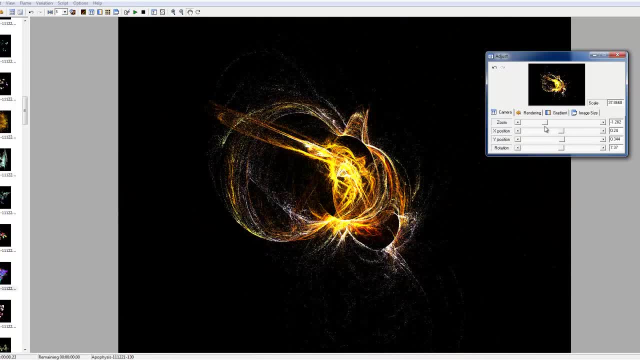 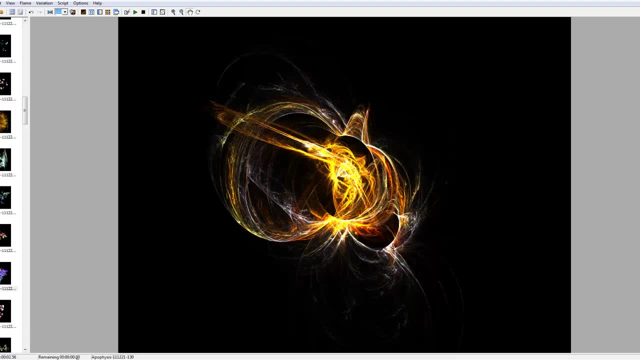 I think, though, I'm going to adjust the zoom just so I can get it all in the picture. First thing we do when we render it Change this back to 100. And, as you can see, it takes a little bit of time. 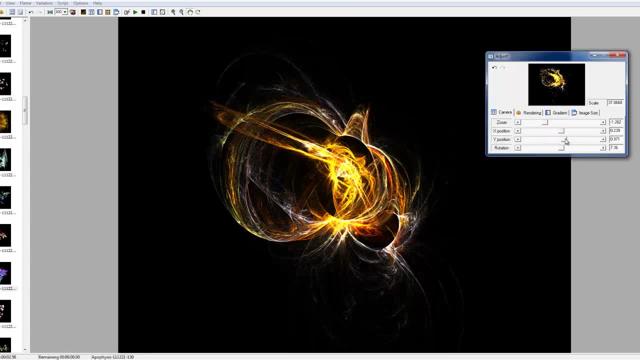 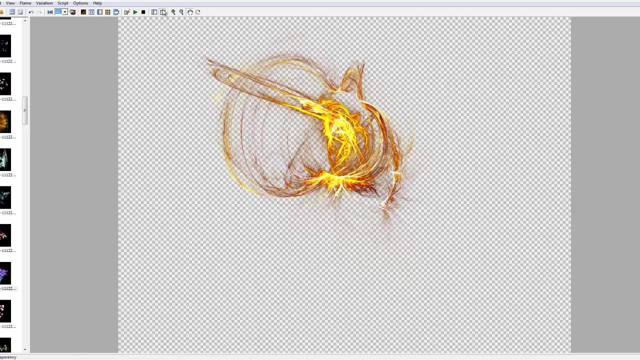 Ooh, I like it All right, So move it up a little bit, just so I can have the whole thing in the frame. Bum, All right, Coolio's Click on that transparency, So it has the transparency there. 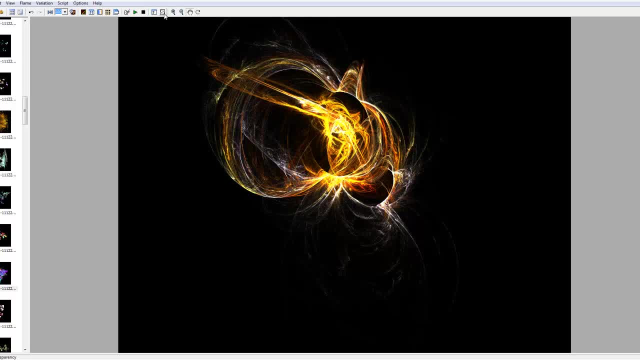 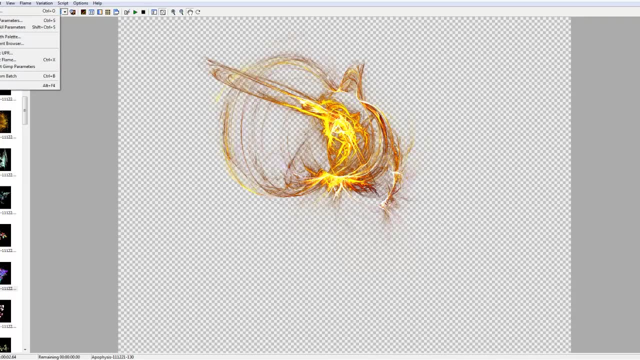 So if you want to use it in Photoshop or something, you can, Because you can just drag it in and slap on a new background, Um, so I'm going to change it to transparency. Then you would think you would go to uh file. 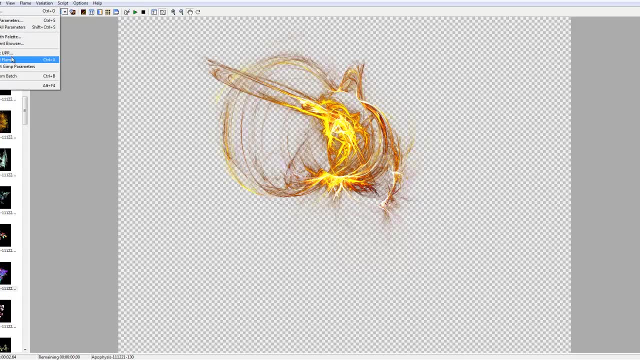 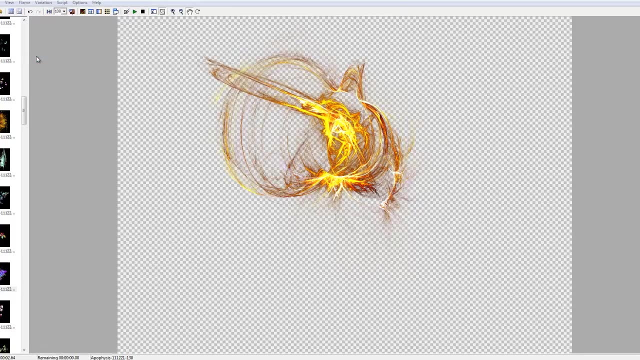 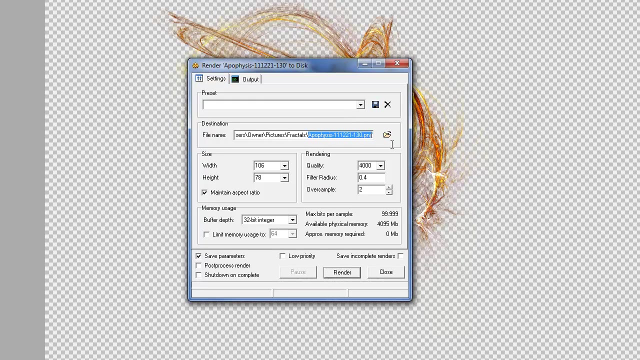 And go to export flame. Don't do that, It doesn't work. Go to flame Right here And click render to disk And it'll bring up this little menu. So I've already got it saved in fractals And you want to make sure you don't delete the png. 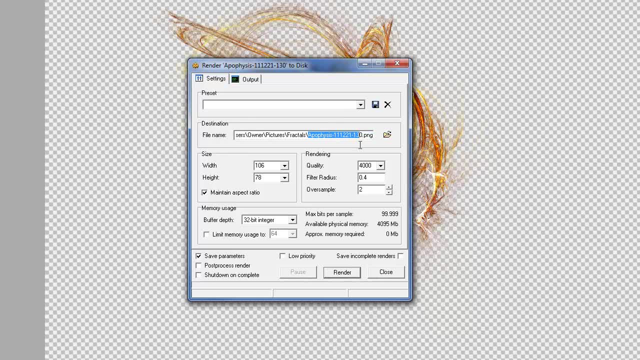 Or else it's going to save it to a different file. It's not good, Sorry about my mic Again. So, Uh, and the different file usually, uh, it's just it. it won't be able to open it or anything. 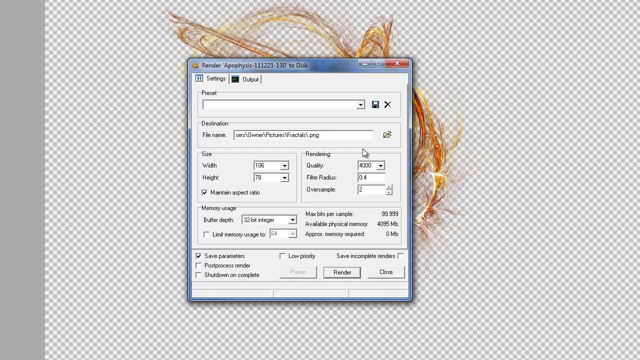 It's just like a blank file. So make sure you don't delete that png, But delete that, The hypothesis and whatever, And rename this. I'm going to name it: YouTube, YouTube swirls, Okay, png. 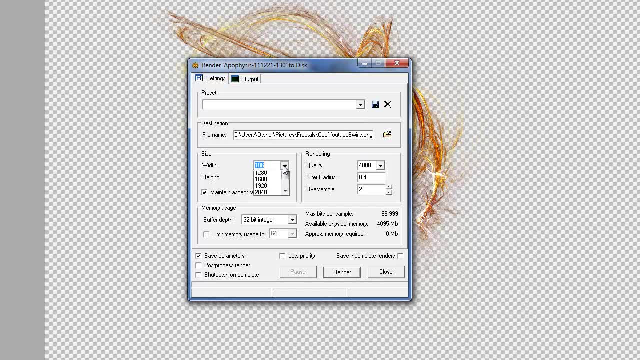 Make sure you have a png extension on the end. It will save your life. Put 920 by 1080.. And it it'll automatically adjust the height. Maintain aspect ratio. If you want to adjust the height yourself, You'll dislike that. 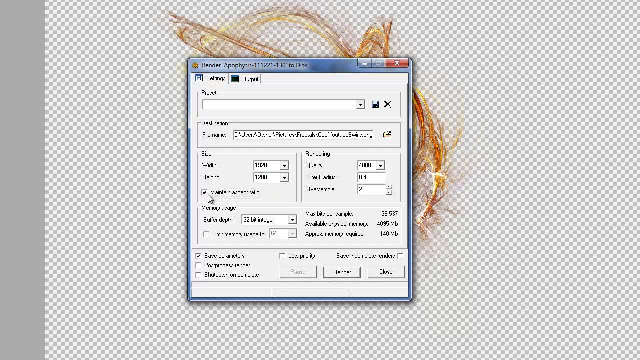 And choose your height To a different, But I want to maintain the aspect ratio: 920 by 372.. Holy crap, Alright, So 920. By 1200.. I suggest to put the quality- It'll be at 200.. 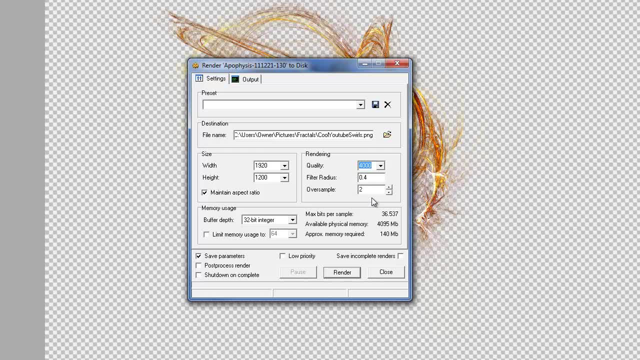 I suggest to put it at 4000.. Just because you'll get superb quality. Uh, and leave everything else. You can play around with that. I haven't done it yet. I just left everything else as it is And it seemed to work. 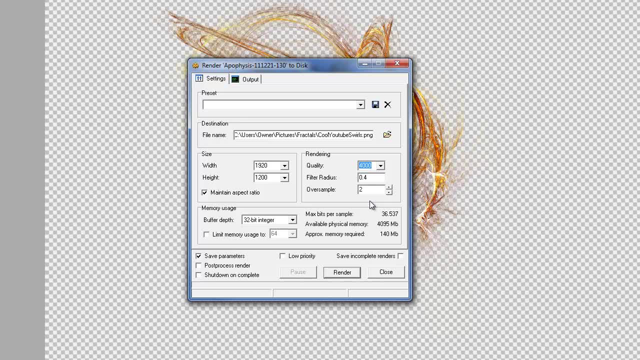 So, um Yeah, 4000.. Now this: I warn you If you don't have a good operating system, Even for my computer, I have 16 gigabytes of RAM And a 6 core processor. It still takes about a half an hour to render this out. 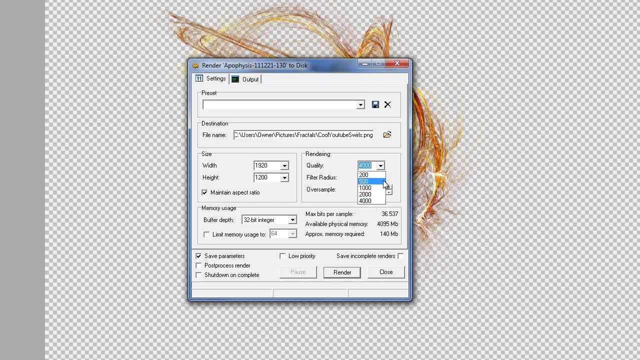 So if you don't want to wait, If you're in a rush, Could do something lower Like 500. But for the purpose of the video I'm going to use 4000. And just pause and restart when it's done. 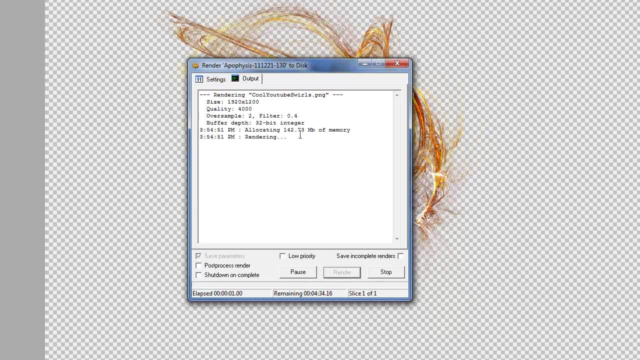 So now I'm going to start the rendering process. It's going to go through. It looks kind of like a DOS program, As you can see. Uh, There's only: Oh, Wow, That's interesting. Okay, Apparently there's three minutes left in this rendering. 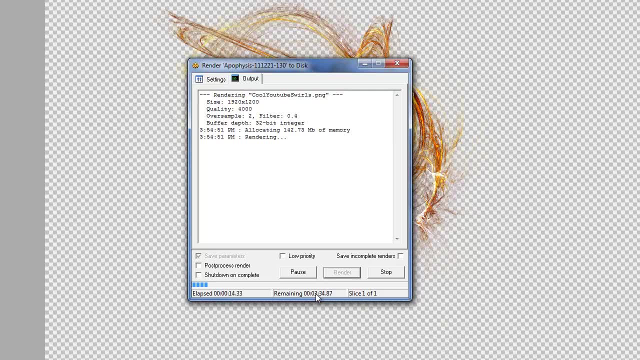 Usually. That's really weird, Because usually it takes me a lot longer, Like a half an hour or so. It might for you, Not sure. So I'm going to pause and restart when it's done: rendering- Alright, So once the rendering process is done, 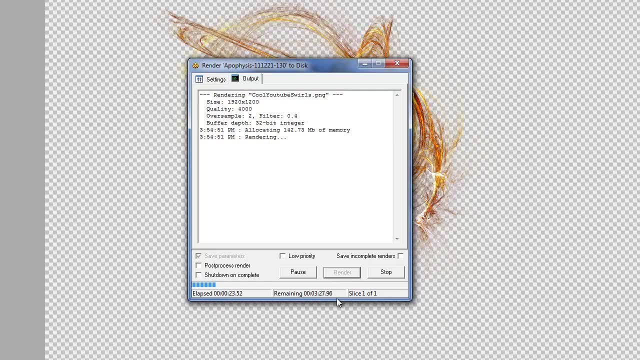 I just finished rendering it out. It's going to run. I don't know. I just need to go and do this. I'm going to run it. It's going to run. I'm going to do this. I'm going to do this. 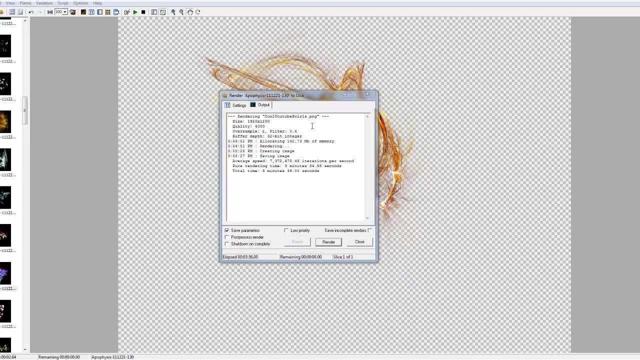 It's going to run. I'm going to do this. I'm going to do this. It's going to run. done? I just finished rendering it out Total time. it'll say your total time, that it took 3 minutes and 36.01 seconds. That's at least what it took me Now. it allocated 142.73 megabytes. 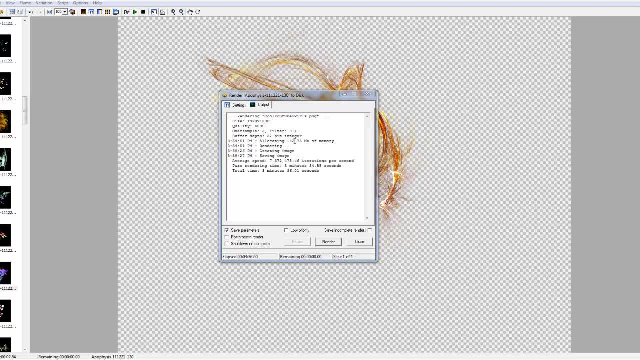 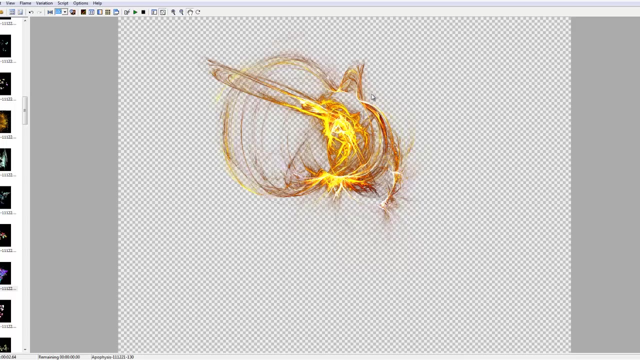 of memory. so if you don't have that- which you probably do, because Windows 7 needs at least 2 gigabytes of memory to run- you'll be fine. So it may just take longer if you only have like 4.. So just close that out or you can press the close button. That is. 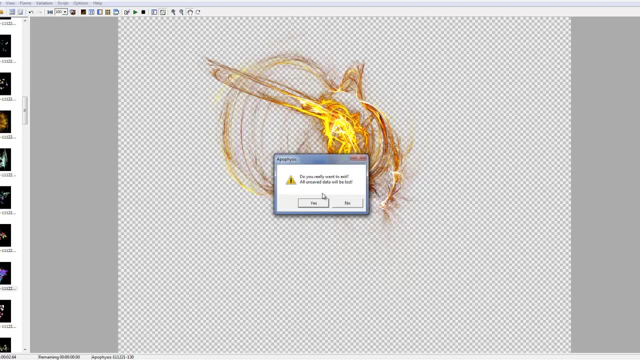 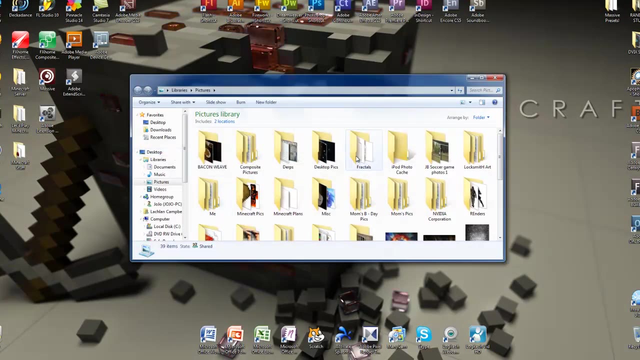 fine as well. Now close this out. If you want to save your data, that's fine. You do that by going up here and say all parameters or say parameters, but I'm not because I don't need it again. Press yes Now, just to make sure we're going to go to my pictures in. 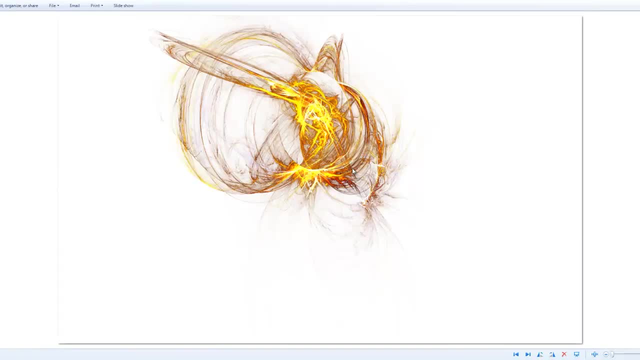 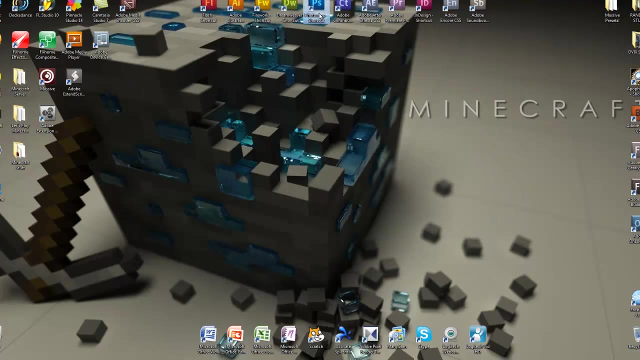 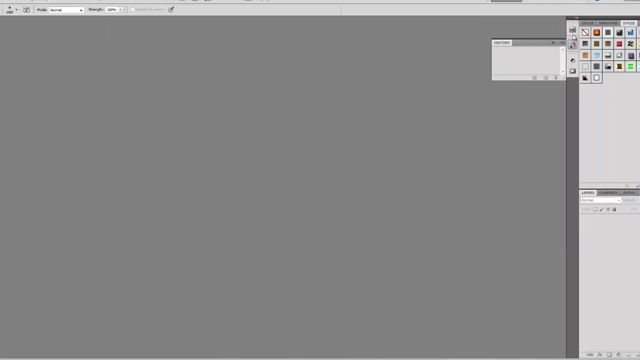 the fractals Cool YouTube squirrel right there. So now you've got the transparency of this cool YouTube squirrel And just to show you that it's a transparency, I'm going to open up Photoshop And I mini bridge there we. 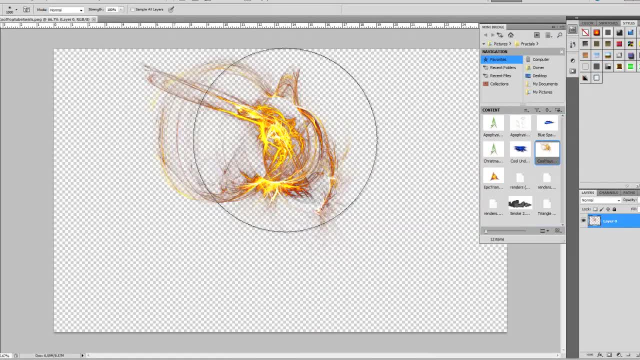 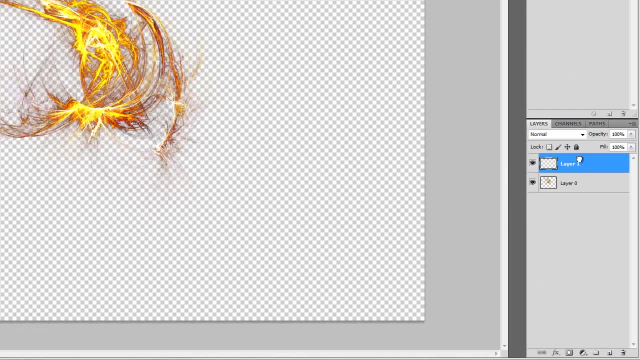 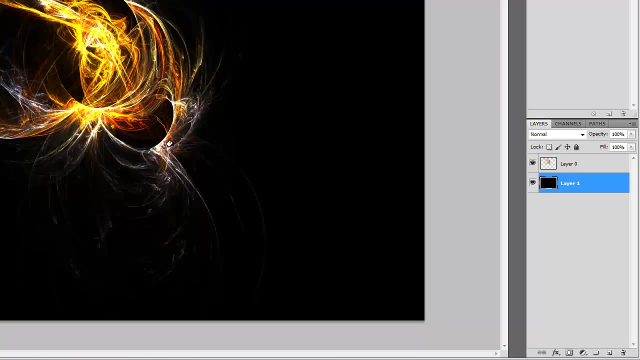 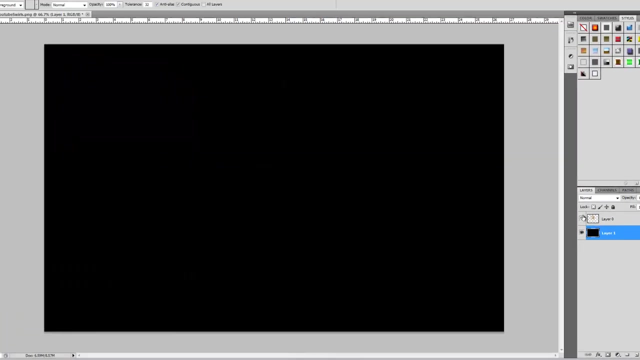 are guys And just drag this on and, as you can see, it is indeed a transparency. Just to prove, or just to prove to you, I'm going to show you how to do it. So I'm going to fill this layer with or not black And see, as you can see, it's very nice, All right. 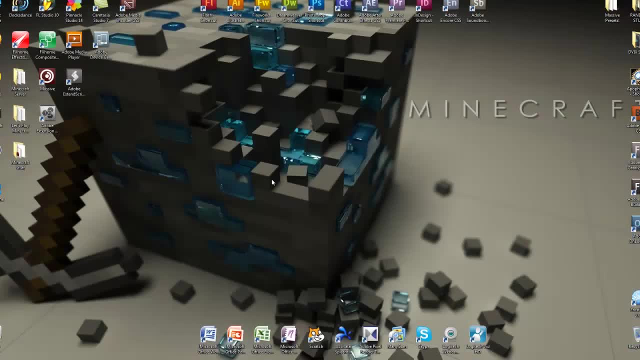 And I hope you enjoyed the tutorial. I'll put a link to this, the picture, the fractal that we created, the transparent version and the one with the black background in the description. Plus, I will put a link to Apophysis. 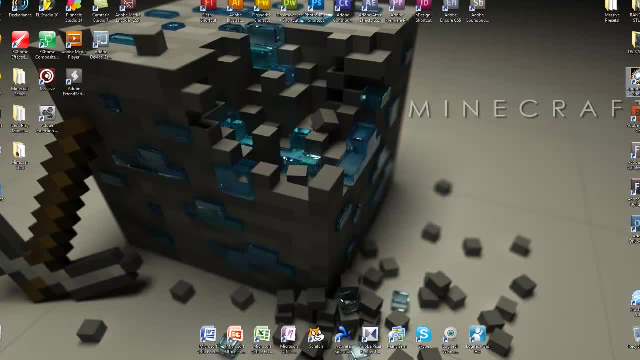 For you, lovely YouTubers, to download. Hope you enjoyed this tutorial. Please rate, comment and subscribe. Especially comment because, if you want to learn more about Photoshop or any of the CS5 collection, Pinnacle Studio, Apple Studio, Minecraft, any other cool softwares- 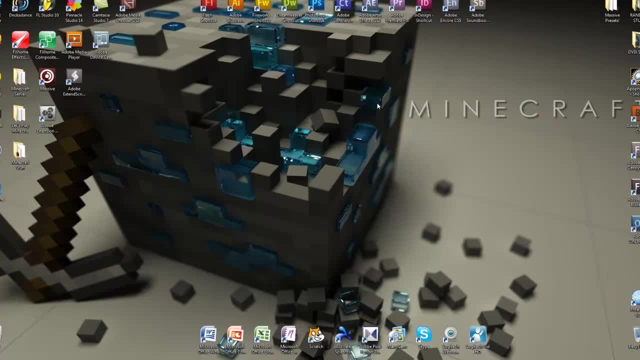 that you want me to check out, please feel free to put in the comment section. I will see you next time, folks. All right guys. So a bit of a side note. Sorry, I've extended this video so long. I just wanted to mention sorry for my mic quality, Probably mentioned in a bunch of other videos. that it's like screwed And I'm broke, so I can't like buy another mic at the present time being. So just bear with my tutorials. As long as they help, that's all that really matters, I think. But just bear with my tutorials. I'll see you next time. Bye.